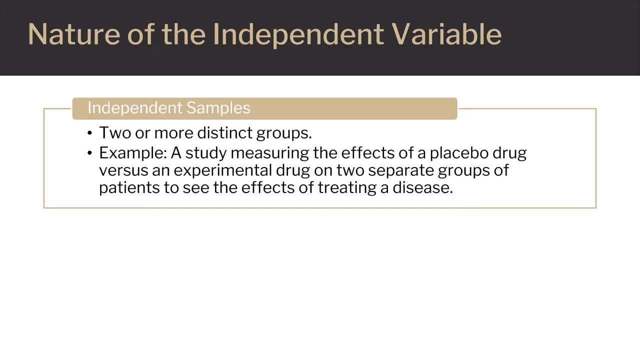 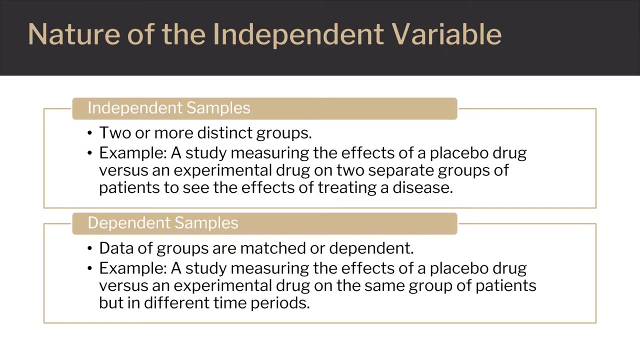 an experimental drug on two separate groups of patients to see the effects of treating a disease. In this example, the two groups have two different groups of participants with different characteristics of each individual within each group. An example of a dependent group is a study measuring the effects of a placebo drug versus. 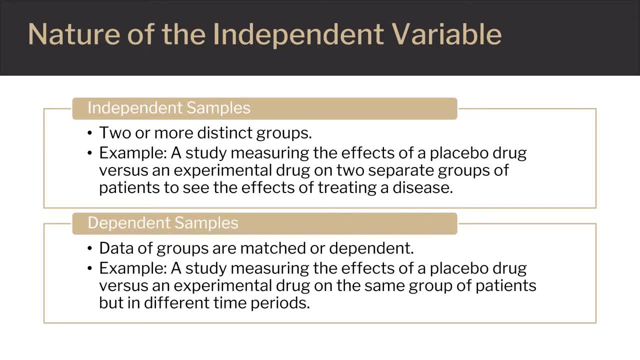 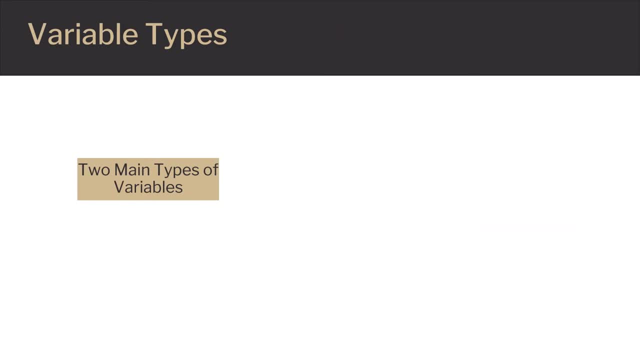 an experimental drug on the same group of patients, but in different time periods. In this example, the two groups that are being studied are the same exact people in each group, but at different time intervals. There are two main types of variables, which are categorical and continuous. 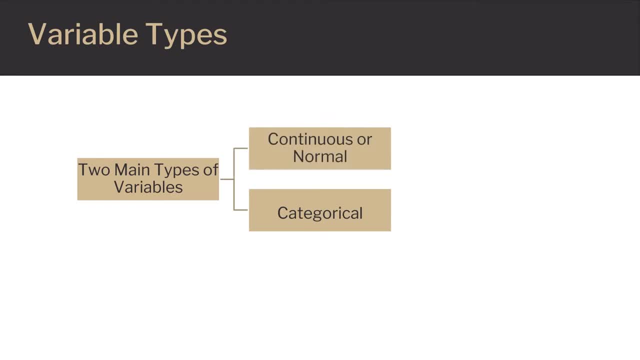 Continuous variables are also known as normal data. Examples include age that is not categorized. For example, you could ask participants what their age is in years, or you could ask them which age group they fall into. Asking which age group they fall into is an example of categorical data. 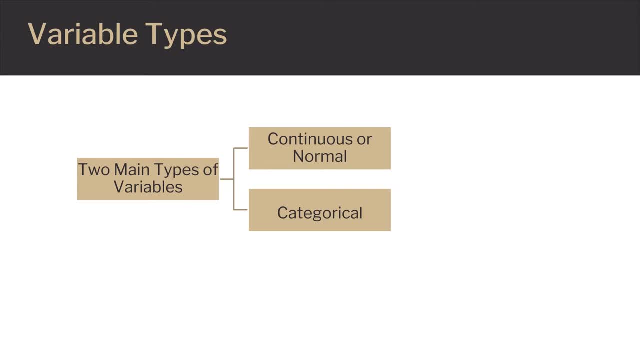 Categorical variables are those that have discrete categories or levels. Categorical data can be further described as nominal, ordinal interval or ratio. Nominal data is categorical. It is categorical in nature but has no specific order, For example, colors such as green, red, blue. they have discrete categories but are in no 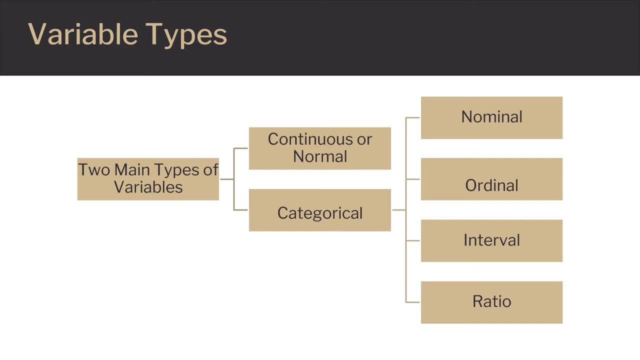 particular order. Ordinal data is categorical in nature, but goes in order. For example, the categories small, medium and large have a clear order in terms of their size. Interval data is categorical in nature and ordered as well, but has well-defined equal intervals. 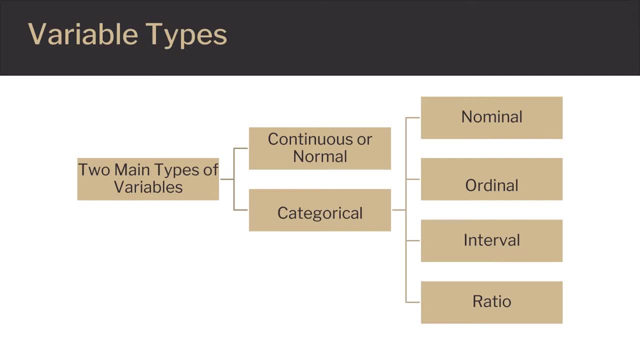 For example, if you were to choose age groups in 10-year intervals, you might group participants from 0-9 years, 10-19 years, 20-29 years, etc. Ratio data is categorical in nature, ordered, has well-defined intervals, but in addition, 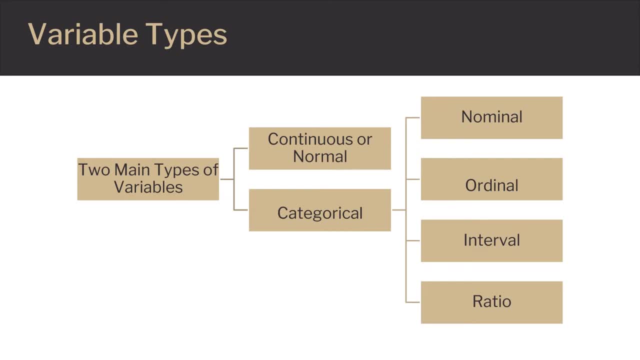 includes the value 0.. An example of ratio data would be age. As we could see in the previous example, you can be 0 years old if you are less than 1 years old, But you need to have data that includes 0 and does not include negative values, so that 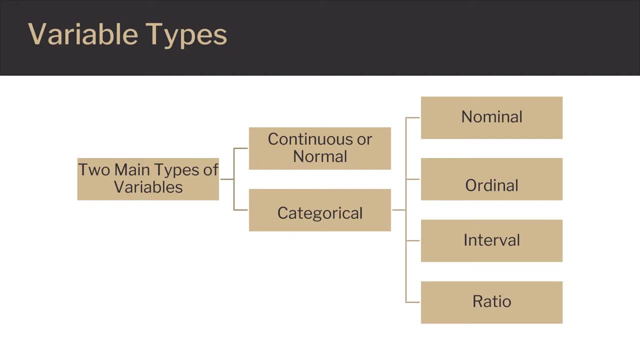 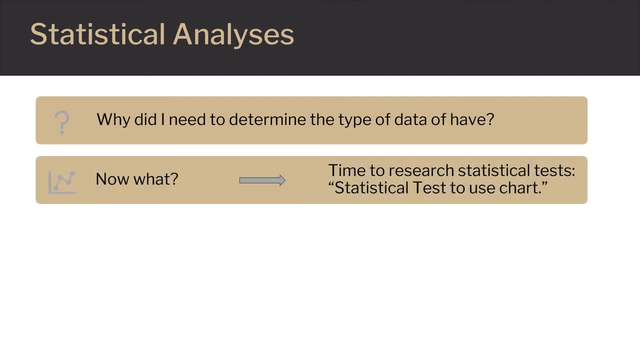 a ratio between two different variables can be calculated. Once you've determined the size of data you have, you can choose the most appropriate statistical test to analyze your data. That's why it's so very important to correctly identify the types of data you have and to 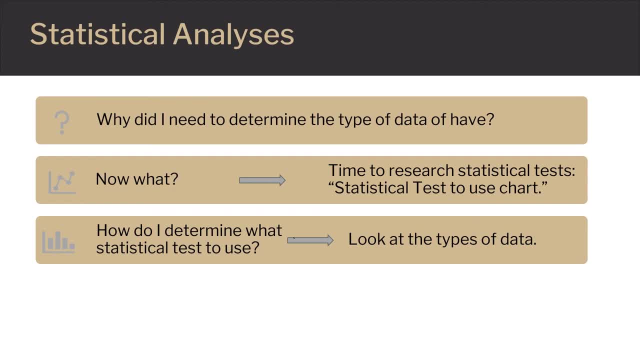 identify which variables are dependent or independent. There are many websites. Using a search engine, you can use the keywords statistical test to use chart To find a chart that is easiest for you to interpret. Once you've determined which statistical test is most appropriate, check to see if. 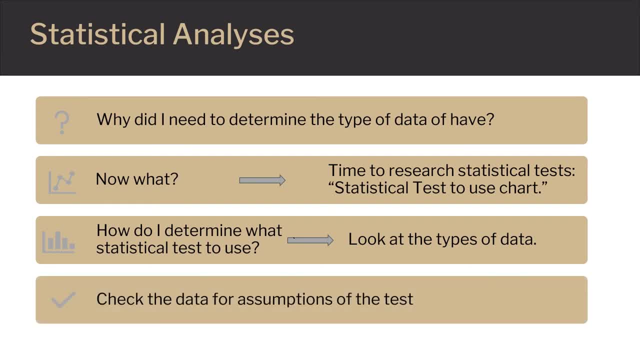 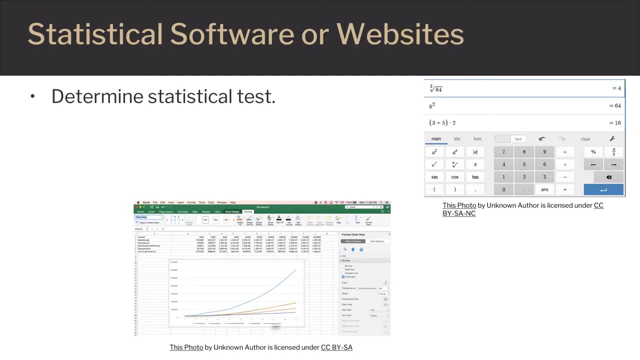 your data meets the assumptions of that statistical test. If the data does not meet the assumptions of the test and it is parametric, such as a t-test, then you may want to research the equivalent non-parametric statistical test, such as the Wilcoxon test. 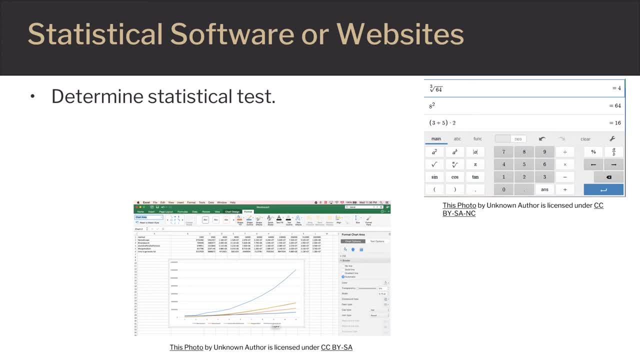 Once you've determined which statistical test you plan to use to analyze your data, you will run the test in either statistical software that you have access to or have purchased. PSPP and R have free public access. Excel is part of Microsoft Office, which is included. as a student of Purdue Global University, 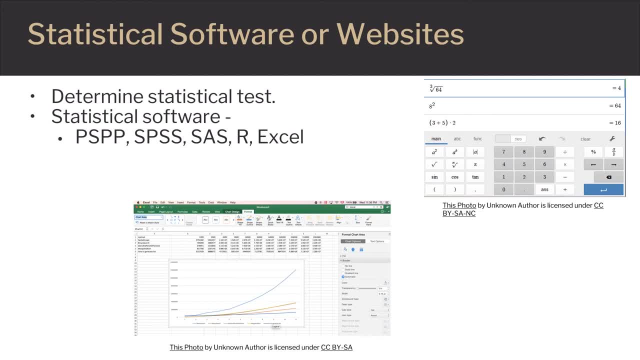 SPSS and SAS are also good programs that can be purchased through the companies. Another way to run a statistical test is to run a test in Microsoft Office. You can run a test in Microsoft Office. A statistical test is to use a search engine and input keywords in your search that contain: 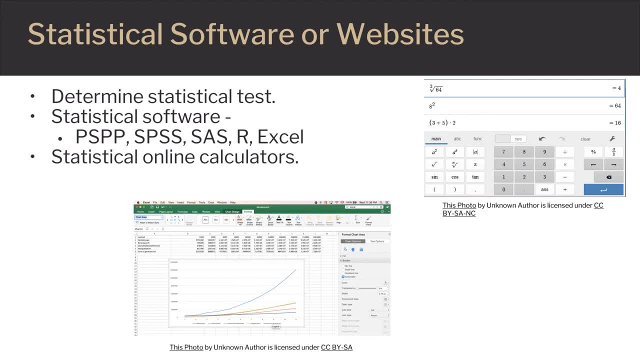 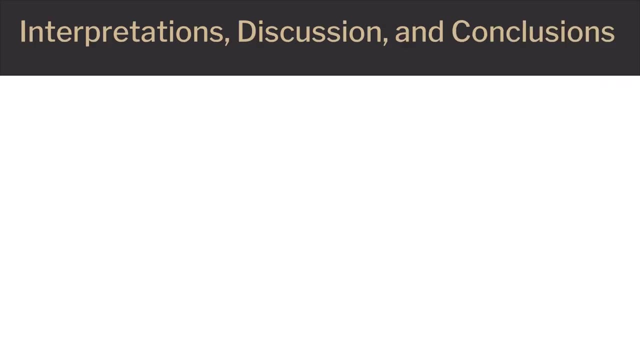 the name of your statistical test, followed by the word calculator. For example, if you want to run an ANOVA, you can type into the search box of a search engine: ANOVA calculator. The sites listed will ask for your data and then will give you a statistical output. 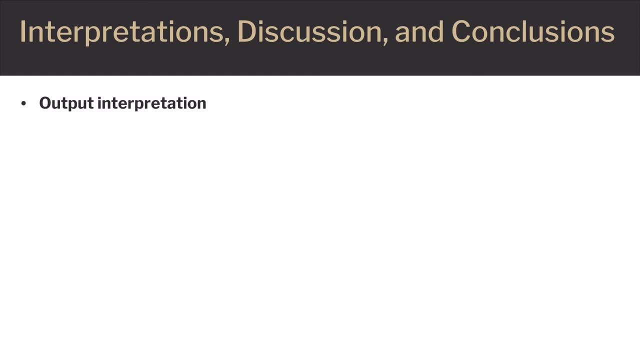 Once you run the statistical analysis, the output, your statistical software or online calculator may be confusing. This is where you should research the interpretation of the output and include the name of the software you used. For example, let's say you're given a p-value of 0.01, where you set the alpha value of 0.05..